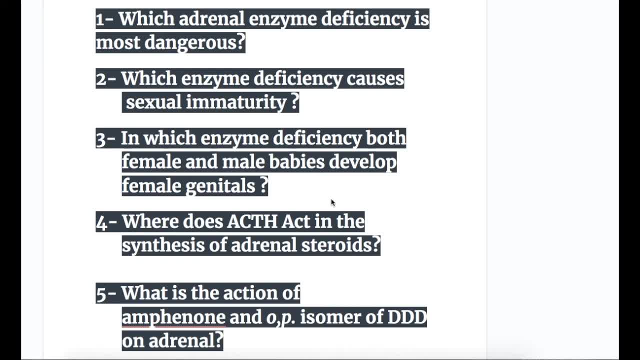 done. Question number one is: which adrenal enzyme deficiency is most dangerous? Number two: which enzyme deficiency causes sexual immaturity? Number three: in which enzyme deficiency both female and male babies develop female genitals? Number four: where does ACTH act in the synthesis of adrenal steroids? Number five: what's the action of amphenone and opdd isomer of ddd? 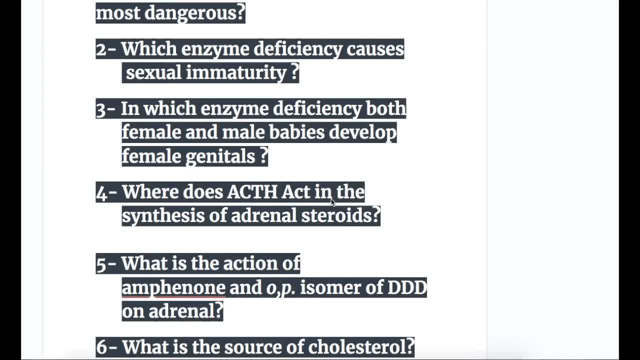 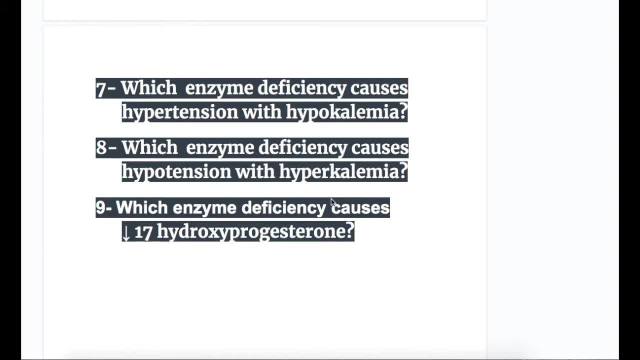 on the adrenal gland. Number six: what's the source of cholesterol? Number seven, which enzyme deficiency causes hypertension with hypokalemia. Number eight, which enzyme deficiency causes hypotension with hyperkalemia. And number nine, which enzyme deficiency causes decreased 17. 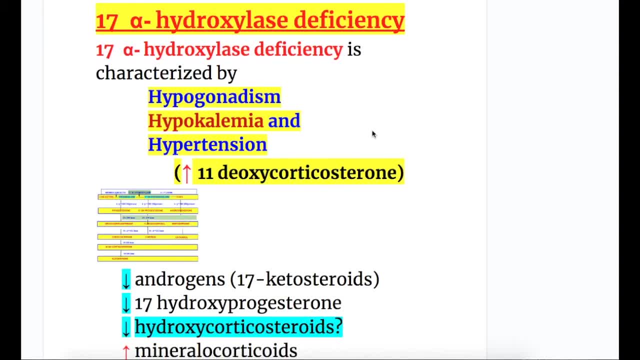 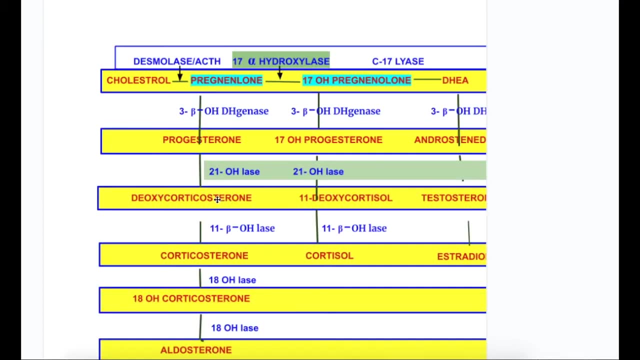 hydroxyprogesterone. Now let's discuss 17 alpha hydroxylase deficiency. 17 alpha hydroxylase deficiency is characterized by hypogonadism, hypokalemia and hyperglycemia. Hypotension. Why hypertension Due to increased deoxycotic oscarones And why there is. 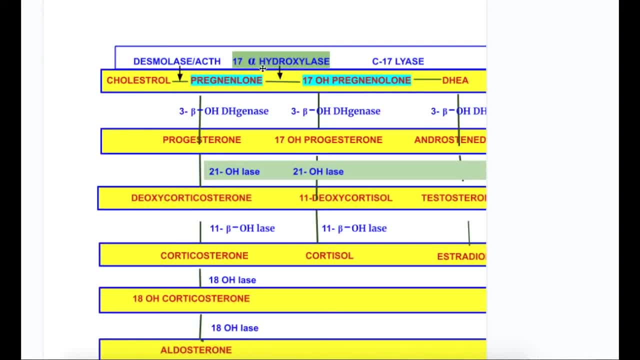 hypogonadism. Let's discuss it here. This is the point where 17 alpha hydroxylase enzyme action converts pregnenolone to 17 hydroxypregnenolone. that is converted to DHEA and androstenedione. 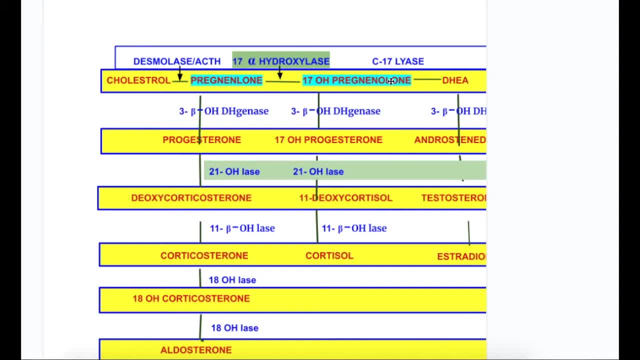 A deficiency in this enzyme, it stops the formation of DHEA and androstenedione. that causes hypogonadism. And number two: this enzyme deficiency causes shunting of the 11 deoxycordisole to deoxycorticosterone, which is a mineralocorticoid. 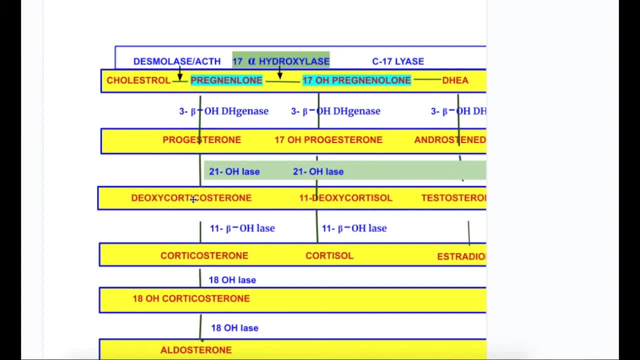 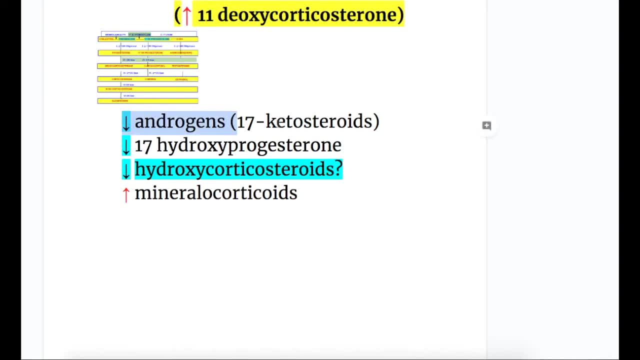 and that causes hypertension with hypokalemia. So, as a result of the deficiency of 17 alpha hydroxylase, there is decreased androgens, 17 ketosteroids, as I already explained, and 17 hydroxyprogesterone, and there is decrease in hydroxycorticosteroids, but there is increase. 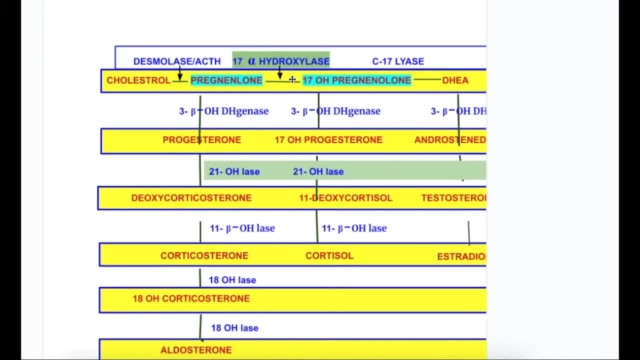 in mineralocorticoids. So if you see here, this deficiency will cause decrease in DHEA and 17 ketosteroids, and also because there is a conversion of 11 deoxycordisole to deoxycorticosterone and that causing hypertension. 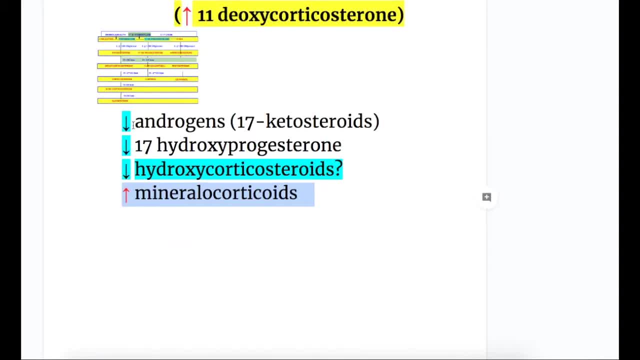 and hypokalemia. So again, these three substances are decreased in 17: alpha hydroxylase deficiency androgens, hydroxyprogesterone and hydroxycorticosteroids. but there is an increase in mineralocorticoids. Other substances which are decreased is decreased. 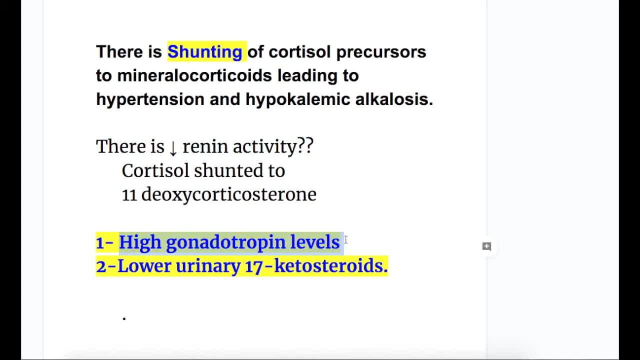 in DHEA and 17 alpha hydroxylase deficiency. Now how is this run? in activity? There is high gonadotropin levels. Why high gonadotropin? Because there is decreased 17 ketosteroids and there are 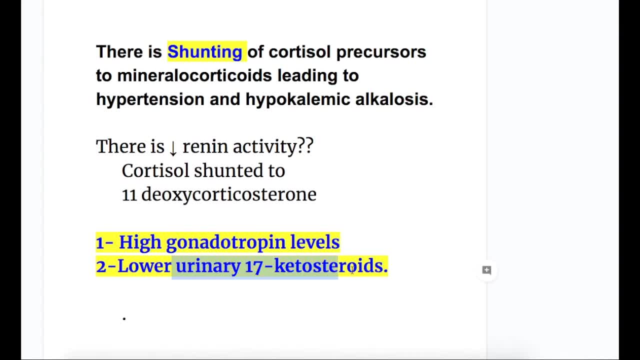 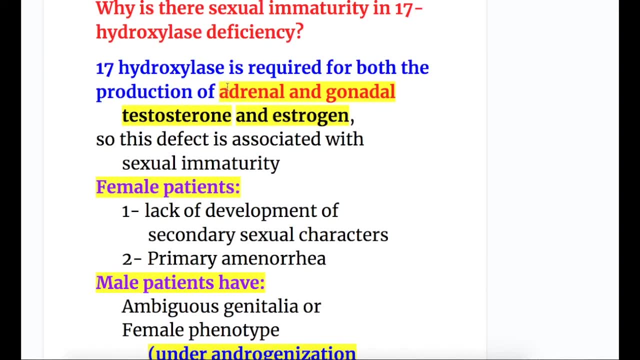 lower urinary 17 ketosteroids. So decreased blood- 17 ketosteroids and decreased urinary 17 ketosteroids with high gonadotropin in 17 alpha hydroxylase deficiency. Why is there sexual immaturity in 17 alpha hydroxylase deficiency? 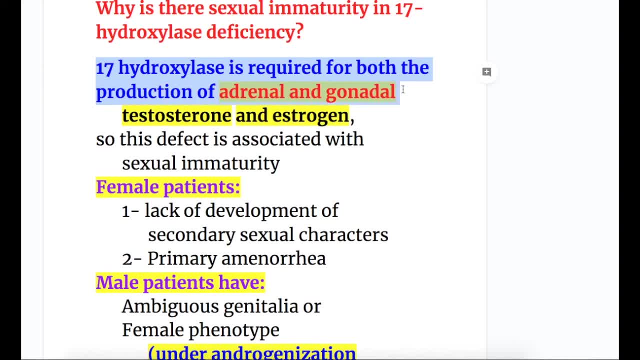 oxylase is required for both reproduction of adenal and gonadal testosterone and estrogen. So this defect is associated with sexual immaturity, because this enzyme is required by both adenal cortex and gonads. So the features in female patients are number one. 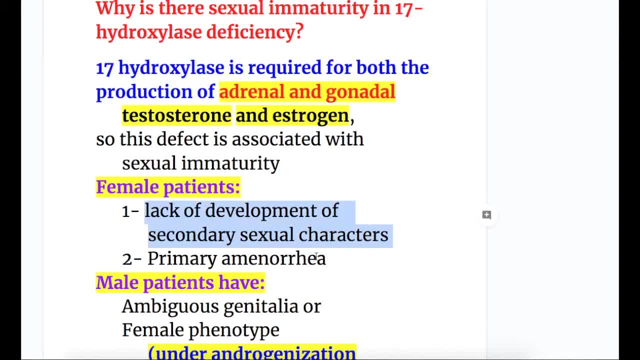 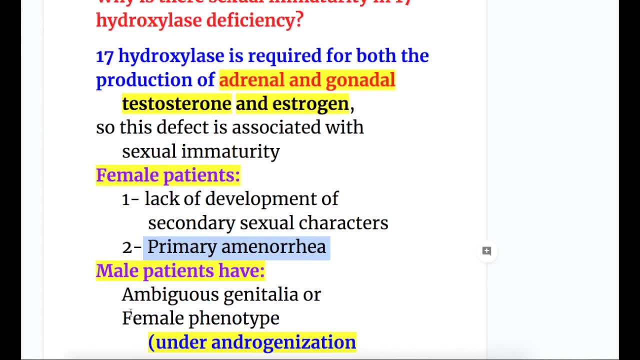 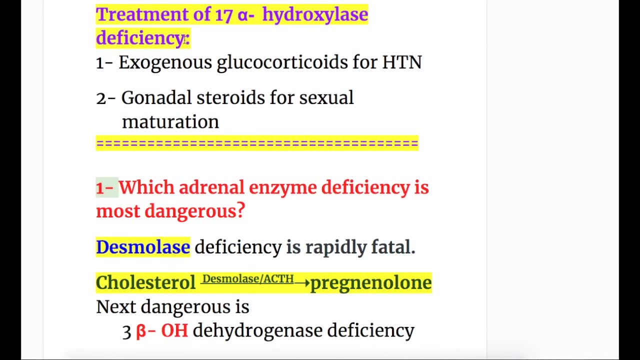 lack of development of secondary sex characters. and number two, primary amenorrhea in female patients And the features in male patients are ambiguous genitalia or female phenotype under androgenization. So what's the treatment of 17-alpha-hydroxylase deficiency? 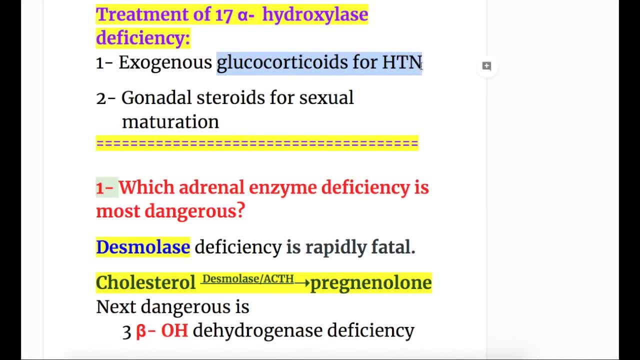 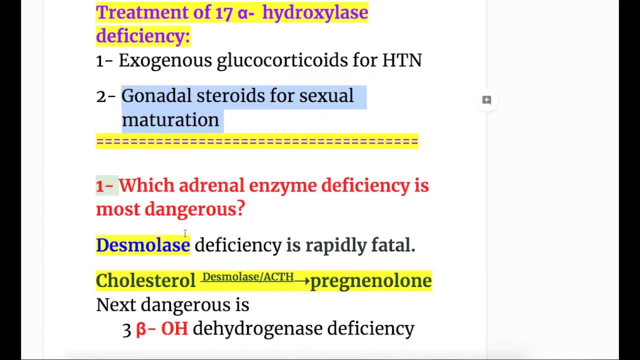 exogenous glucocorticoids for hypertension and gonadal steroids for sexual maturation. Now answers to the questions: Which adenal enzyme deficiency is most dangerous? Desmolase deficiency is the most dangerous and is rapidly fatal. So where does desmolase deficiency come from? It comes from the genital cortex, So where does 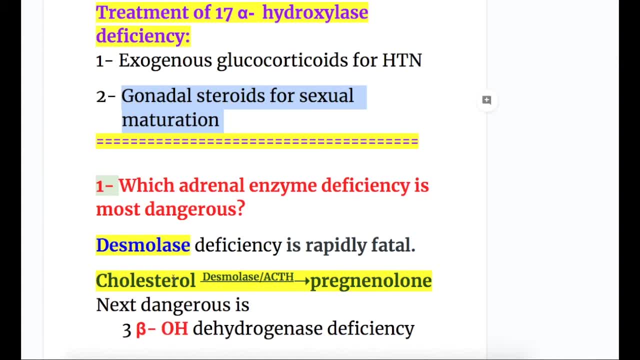 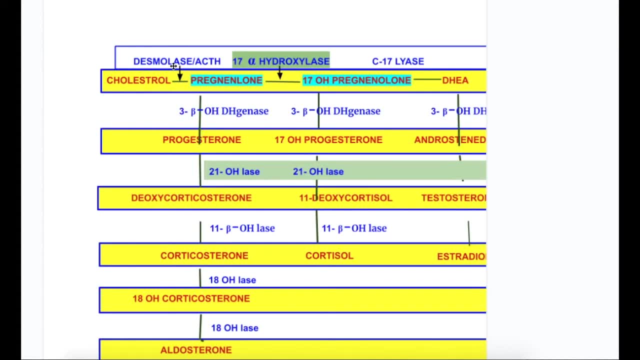 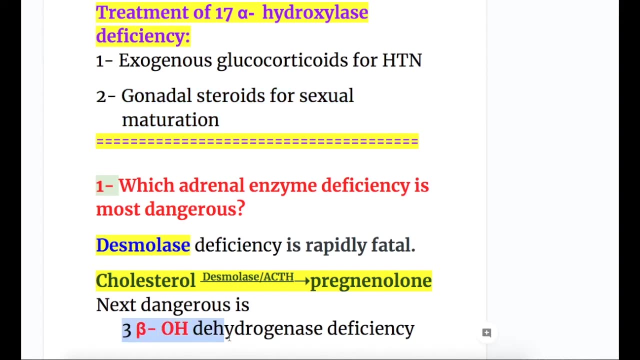 desmolase X. Desmolase X when cholesterol is converted to pregnenolone. in the first step, As you see here, cholesterol is converted to pregnenolone by reaction of desmolase. A deficiency of desmolase is rapidly fatal And the next dangerous is 3-beta-hydroxylase. 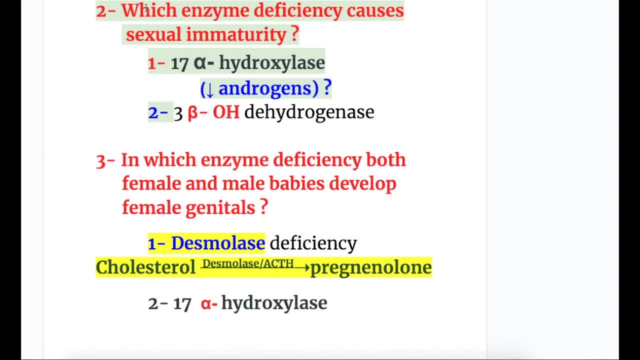 dehydrogenase deficiency. Which enzyme deficiency causes sexual immaturity? Number one: as I already mentioned, 17-alpha-hydroxylase deficiency causes sexual immaturity Because there are decreased androgen production. And number two: it is also required by gonads for 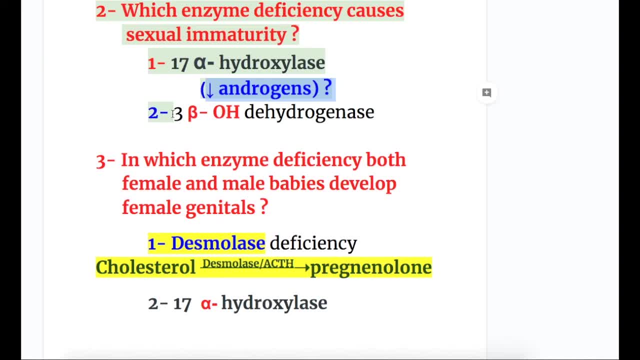 steroid synthesis. And second enzyme that causes sexual immaturity is 3-beta-hydroxylase dehydrogenase deficiency, Because this enzyme is also required for the formation of steroid hormones in the gonads. Question number three, in which enzyme deficiency both female and male babies develop. 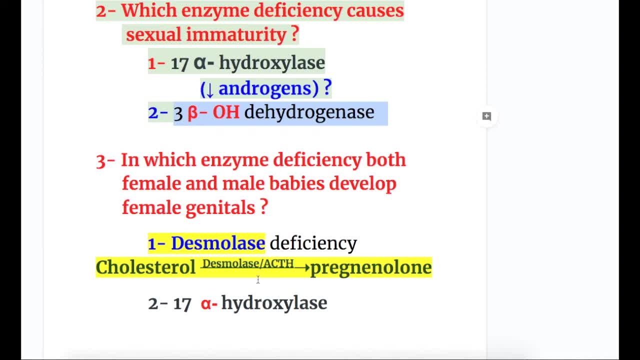 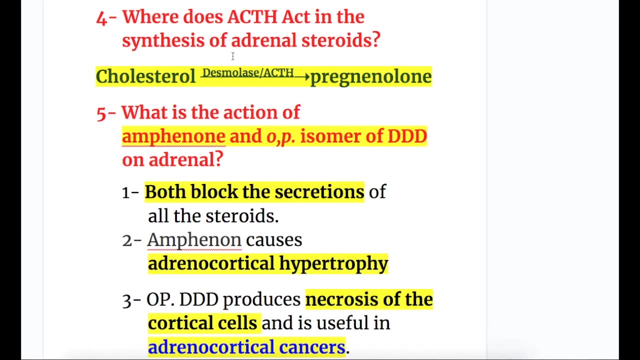 female genitals? The answer is desmolase deficiency. As I already mentioned, acts on conversion of cholesterol to pregnenolone And number two, 17-alpha-hydroxylase, also required for steroid synthesis in gonads. Where does ACTH act in the synthesis of adrenal steroids? 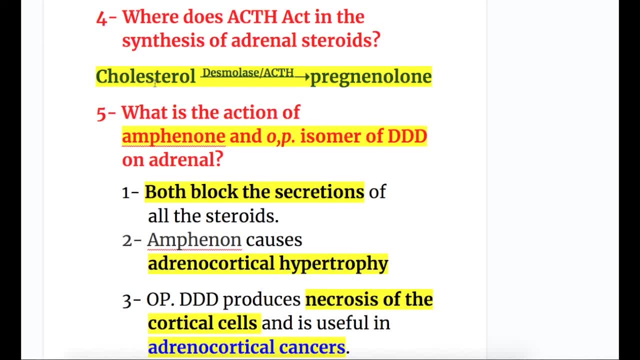 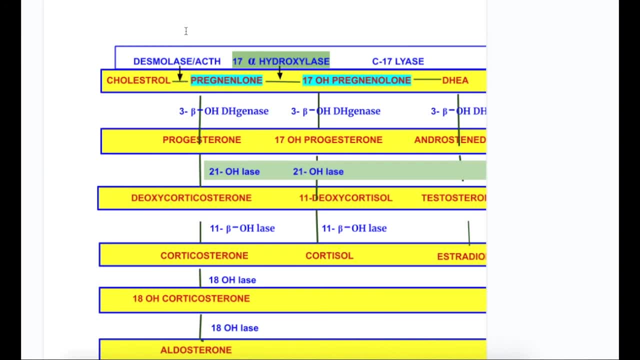 It acts also on the same step for the conversion of cholesterol to the pregnenolone. It is the first step where ACTH act in the synthesis of adrenocortical steroids. What's the action of amphenone and OP isomer of DDL? It acts on the conversion of cholesterol to pregnenolone. 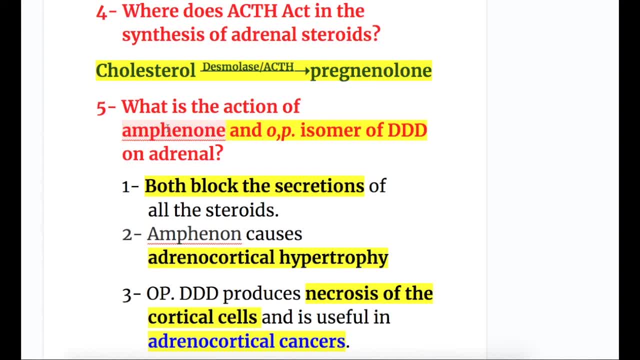 Both these substances, amphenone and OP, isomer of DD, block the secretions of all steroids. Number two, amphenone, causes adrenocortical hypertrophy, And number three, OP-DDD, produces necrosis of the cortical cells and is useful in the treatment of adrenocortical cancers. 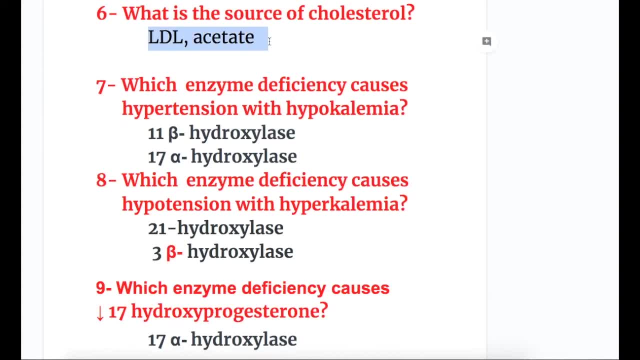 What's the source of cholesterol, Low-density lipoprotein and acetate, And which enzyme deficiency causes hypertension with hypokalemia? 11-beta-hydroxylase and 17-alpha-hydroxylase: These two enzyme deficiency causes hypertension. 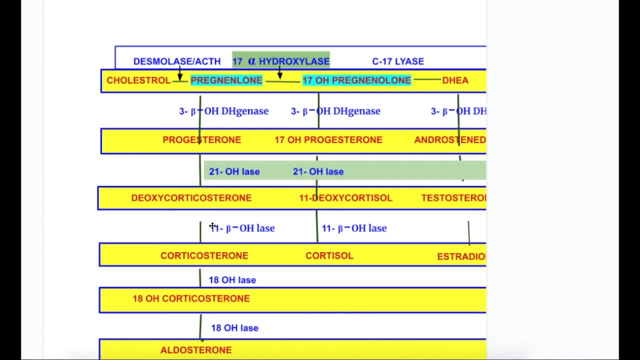 with hypokalemia, As I already mentioned, when this 11-beta-hydroxylase is deficient, so there is increased formation of deoxycorticosterone. Similarly, when 17-alpha-hydroxylase is deficient, there is shunting of 11-deoxycortisol to deoxycorticosterone, So both of them causing 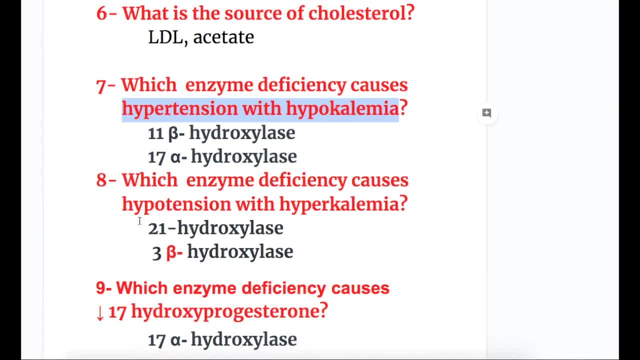 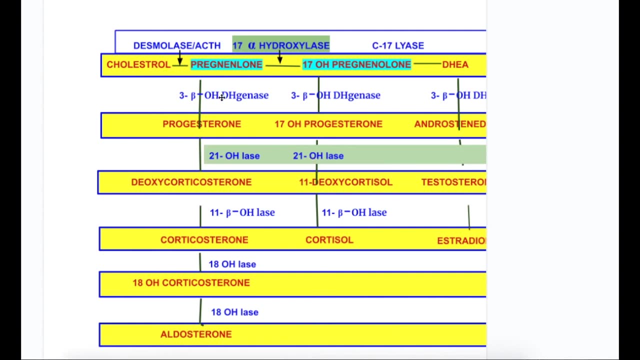 hypertension with hypokalemia. Number eight: which enzyme deficiency causes hypertension with hyperkalemia? Two enzymes, 21-hydroxylase and 3-beta-hydroxylase deficiency cause hypertension with hyperkalemia. See here these two enzymes: if 3-beta-hydroxylase dehydrogenase and 21-hydroxylase dehydrogenase.